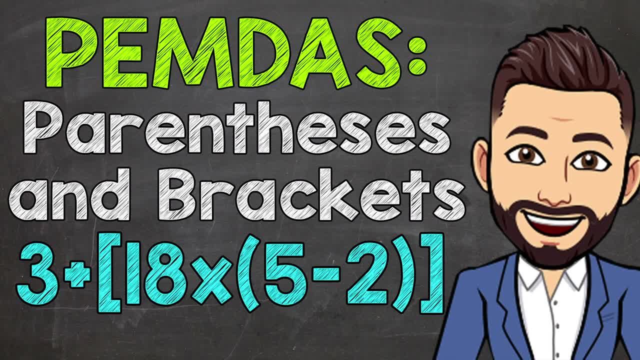 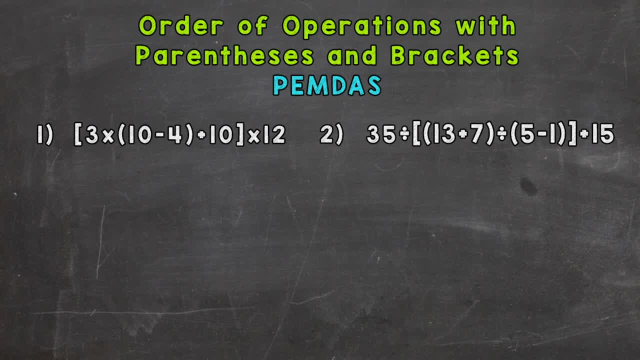 Welcome to Math with Mr J. In this video we're going to take a look at order of operation, problems with parentheses and brackets, or multiple sets of parentheses, and you'll sometimes hear these problems called nested parentheses problems, which just means parentheses within parentheses or brackets. So, as you can see on your screen, we have number one and number two and these are the. 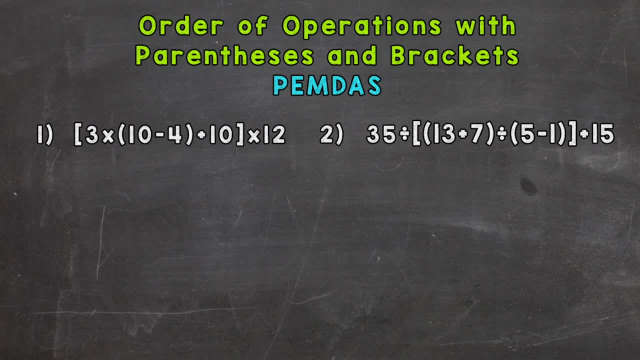 problems we're going to go through together in order to get this down. So let's take a look at number one here, where we have a set of brackets and then parentheses within those brackets. So, just like any order of operations problem, we're going to use the PEMDAS steps Parentheses. 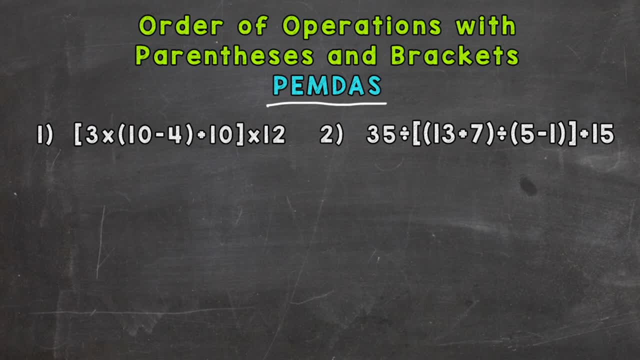 exponents, multiplication and division, and then addition and subtraction. So whenever you see brackets, this is the same. they hold the same value as parentheses. They are priority number one. So this problem has a set of brackets. so the first thing we're going to do is solve everything within those brackets. 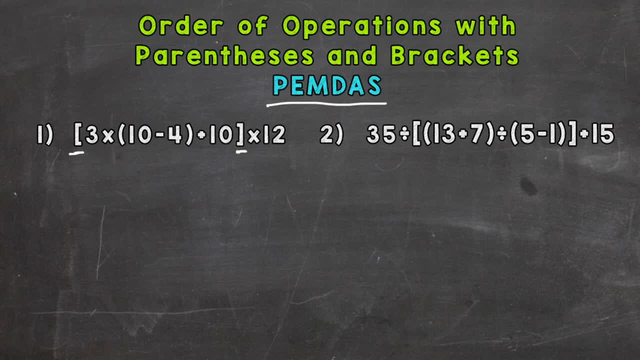 So it's almost like a separate problem, It's a problem within a problem. So we have three brackets and then we have a set of brackets, and then we have a set of brackets, and then we have three brackets, and then we have a set of brackets, and then we have a set of brackets, and then we have. 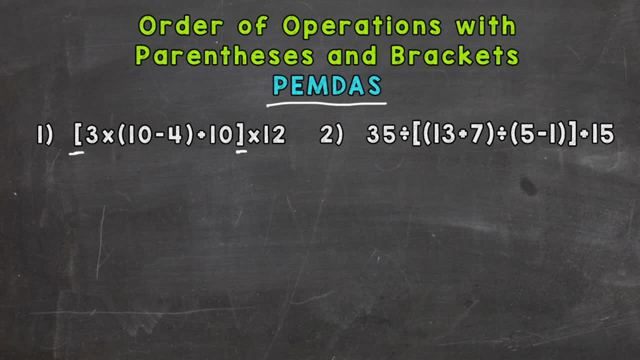 three times 10 minus 4, in parentheses, plus 10.. So we need to go through our PEMDAS steps within those brackets. So do we have any parentheses? Yes, So that's what we do first. 10 minus 4 gives us 6. 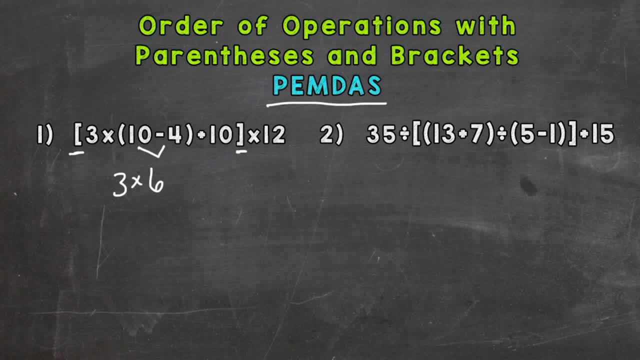 and we can bring down everything we did not use yet, including those brackets. and we're just going to break this problem down one step at a time. So let's take a look at number one. So we have one step at a time. So next, within the brackets, we have 3 times 6 plus 10.. So any more parentheses? 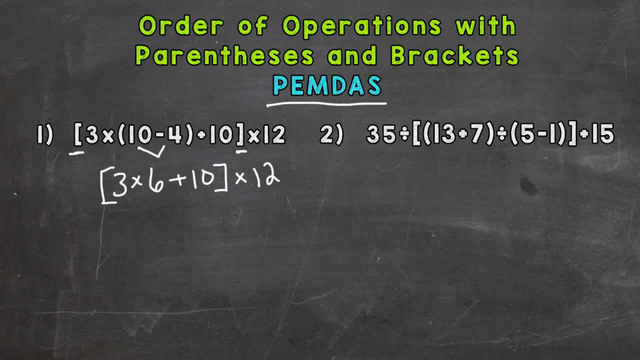 No, Any exponents. No Any multiplication or division. Yes, So that's what we're going to do next: 3 times 6 is 18, and bring down everything we did not use, including the brackets again. Now we're left with just addition within those brackets. So that's what we need to do next: 18 plus 10. 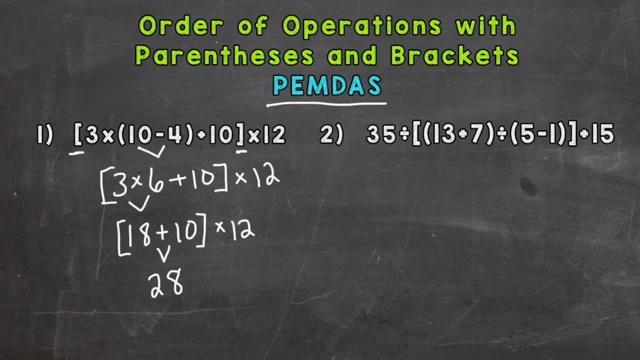 is 28.. Now that we solved everything within the brackets and there are no operations left, the brackets are gone and we can bring down our multiply by 12.. And lastly, we have 28 times 12, which gives us an answer of 336.. So these problems look big and intimidating at first, but if you just break them down one step, 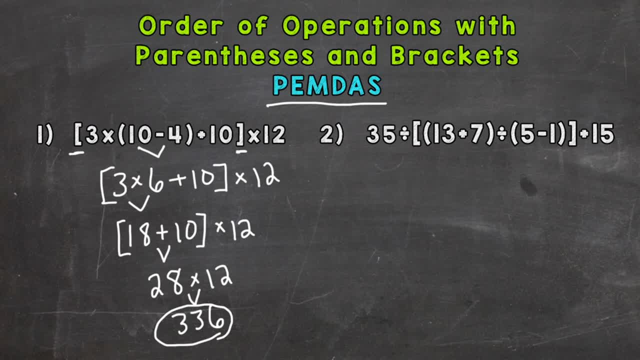 at a time, they're really not too bad. So let's take a look at number two, where we have another set of brackets, like number one, but here we have two sets of parentheses within the brackets. So let's start breaking this down. Remember, inside the brackets this is almost like a separate problem, so we're going to worry about. 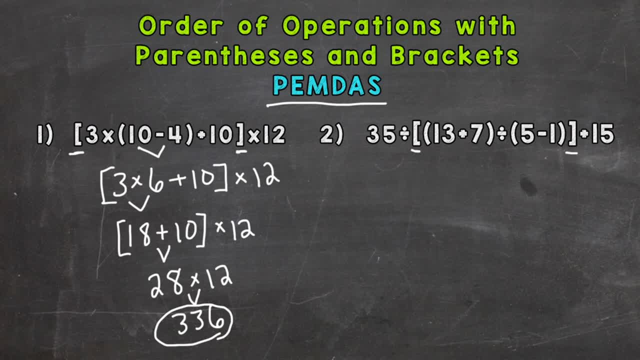 inside the brackets, first break that down and then worry about outside. So here we have 13 plus 7 in parentheses divided by 5 minus 1 in parentheses. So two sets of parentheses So both priority level number one here. so we need to go left to right. So 13 plus 7 gives us 20.. 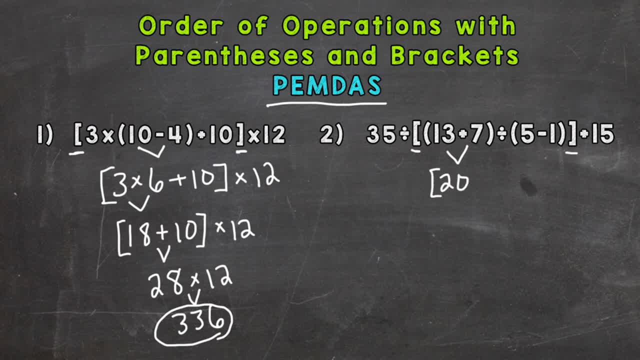 Now we can bring down everything We didn't use and start to break this down further. and 35 divided by, So now we have 20 divided by 5 minus 1.. So parentheses come next and bring down everything we did not use, including the brackets, The. brackets will go away until we get to 20.. For the brackets its only one set of 10, hundred dollars, So forars are across forever. So that gives us 3, assuming already explained by equal maddie accurate, and that is sufficient. You can now look, we can put the 크 age.